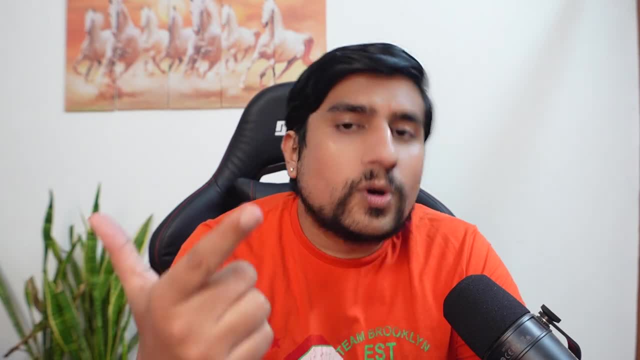 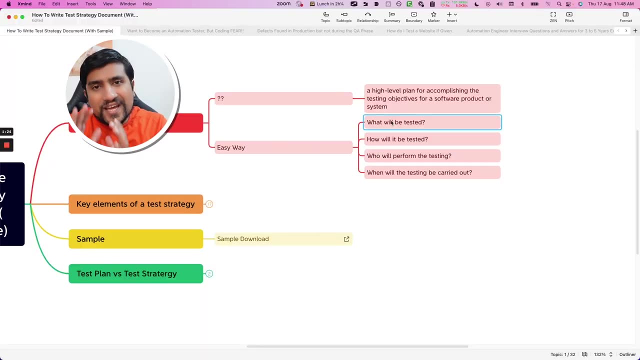 level plan. In this plan, what you need to mention is what and how you are going to do the things, which is how you are going to test what you are going to test what not. You are going to test So easy way. if you want to explain in an interview, right, what exactly you. 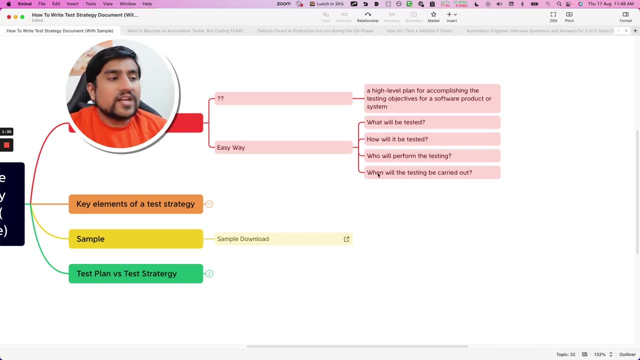 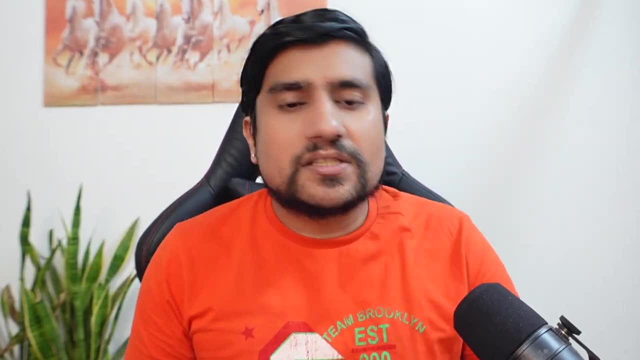 want to test, how it will be tested, who will perform this testing and when it will be basically carried out. All these are basically answered: What, how, who and when. That's it in this case. For example, consider this scenario: I have an e-commerce website, For example, I have amazoncom. 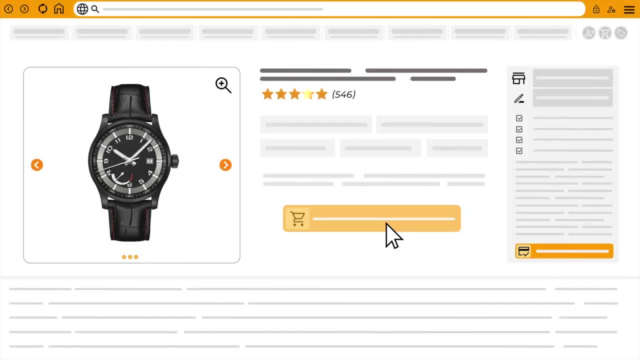 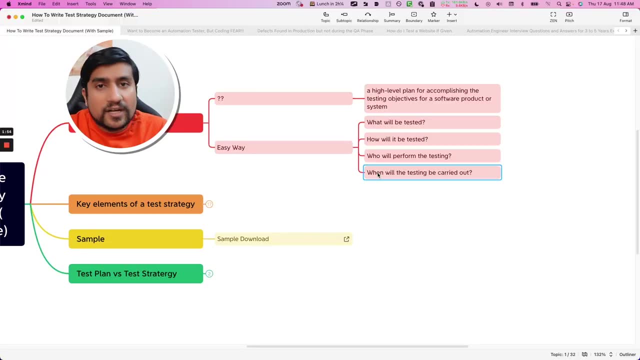 where we have registration page, login page, product listing page, order page and payment processing page, right. All these, basically, are here. So how you can basically create the most important thing for this kind of project, how you can create a strategy right, Let's see that So. 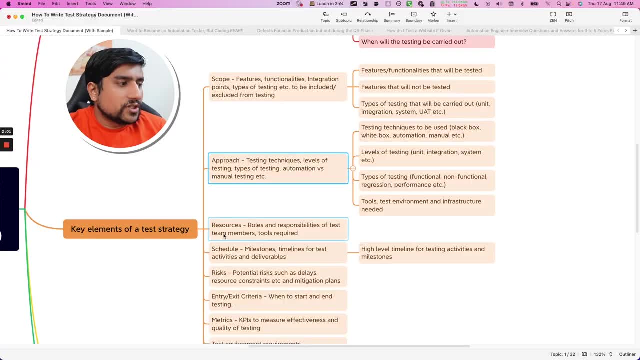 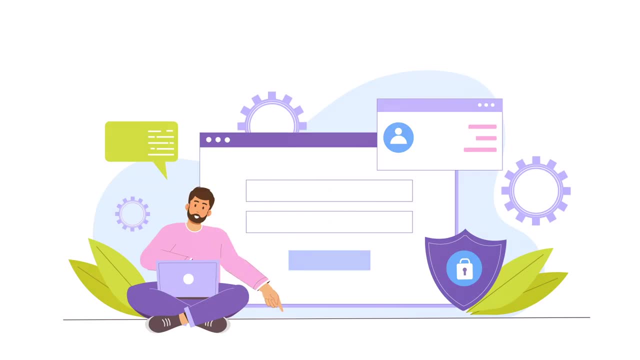 key elements. Key elements involve around, basically, scope. what will be your approach, your resources allocation, scheduling, risk, exit criteria, matrices, test, environment, regression approach. In the scope, you will basically mention what are the feature and functionality that you are going to test, What are the feature and functionality which are out? 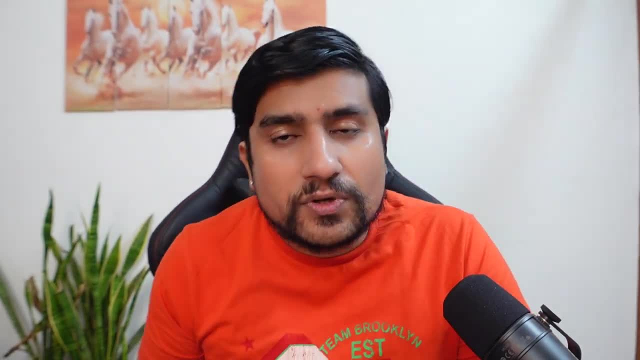 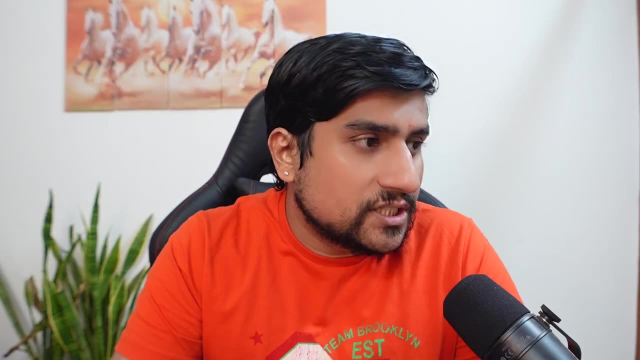 of scope, All these you are going to mention What type of testing you are going to do. For example, you are going to do unit testing integration system, UAT, everything you are basically mentioning How you are going to design your test cases, which is blackboard testing technique. 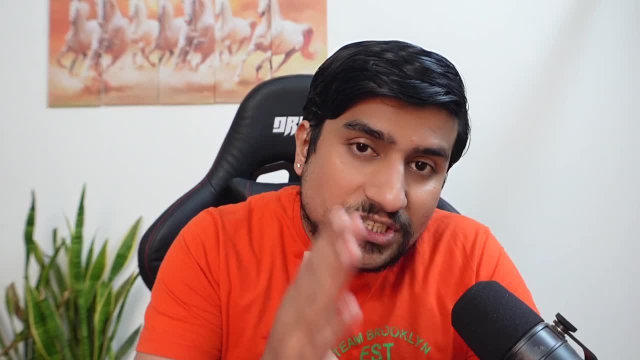 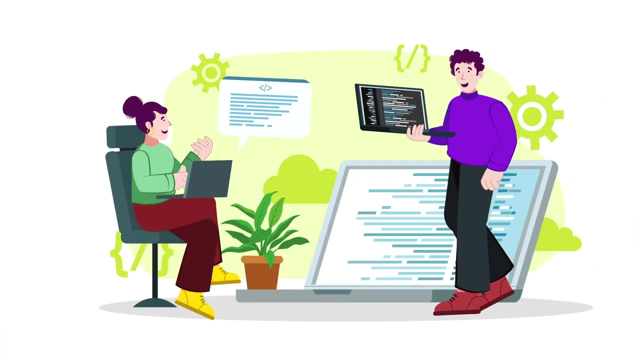 automation, you are going to do manual, you are going to do All these things. you will mention The different levels, for example, unit integration and system, All information on this. Not only that, you will mention right, if you are going to do only functional testing, or are you going to do? 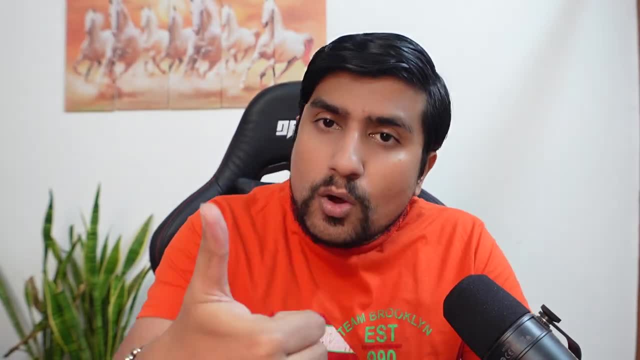 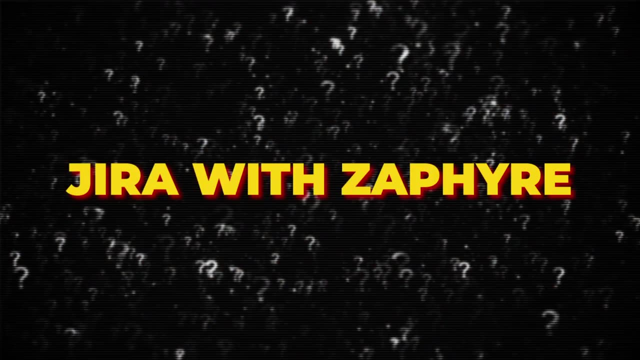 non-functional also, where you are going to do performance testing, security, load compatibility and any other approach. also. You are going to mention everything, Which tool you are going to use. for example, are you going to use Jira with Zafire- Zafire is a test management tool- or you? 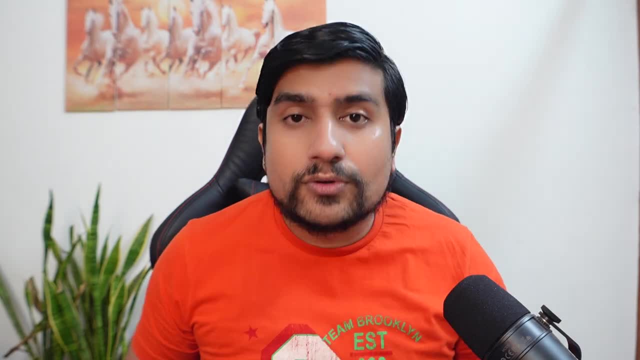 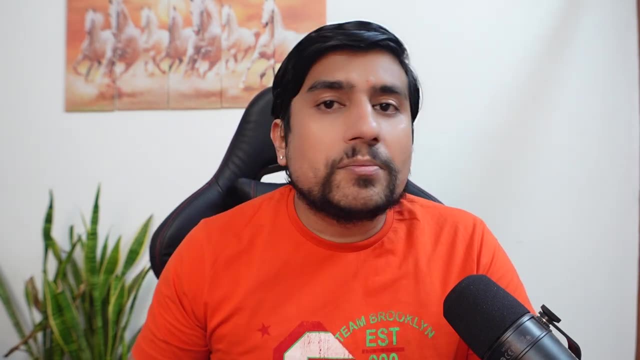 are going to use Bugzilla with the test link, Any open source tool you are going to use? All these you need to mention here Which environment you are going to use. Are you going to use QA environment, pre-prod environment? What environment you are going to use and what are the infrastructure. 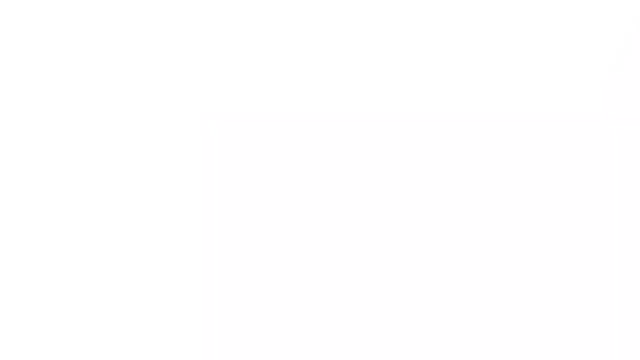 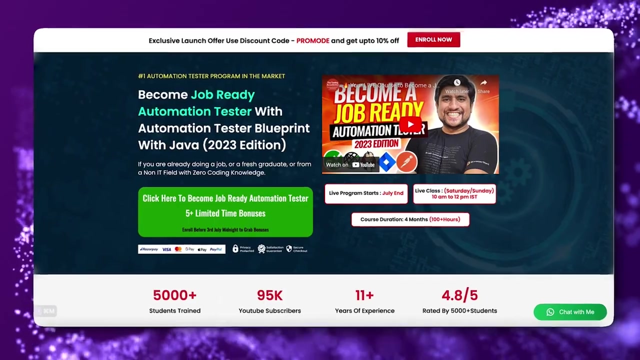 needed right. What are the branches? Everything you will generally mention in this case, Automation is the need of the hour. This is a wake-up call for the manual testers. If you want to convert to automation, job ready automation tester batch is now live. Four months live batch: Saturday, Sunday: 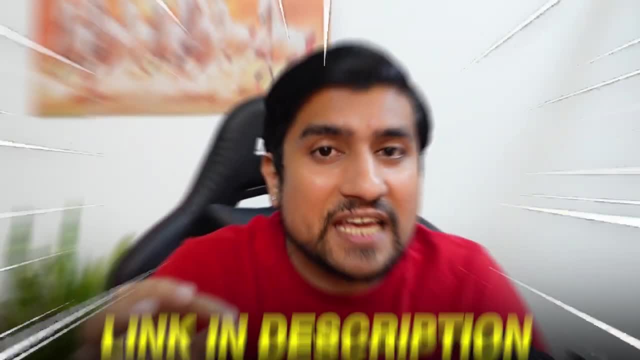 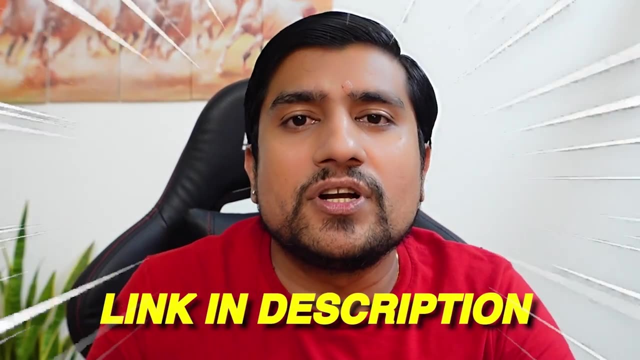 we are going to learn about core java, api automation and web automation. Link is in the description. You check it out. All the projects are live Will be 24: 7 doubt sessions on sdclub. Check out the more details. Not only that, I remember that you are going to see a lot of. 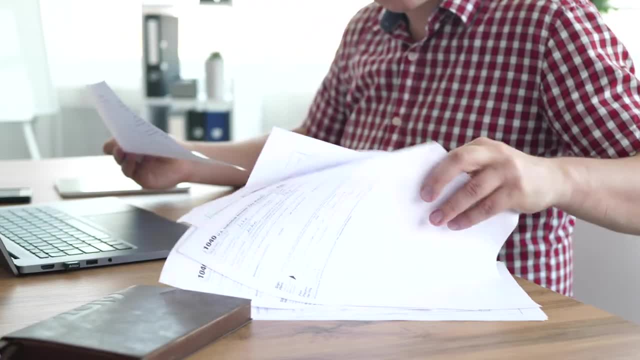 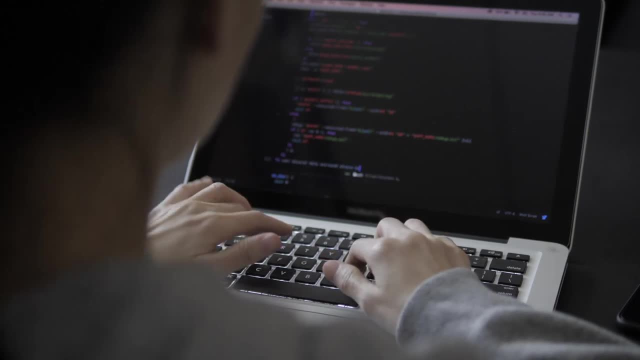 bugs. I also mentioned what are the resources we are going to basically use. What are their responsibilities? For example, junior QAs like me. we are going to write test test cases and execute the test cases. QA lead will write the test plan and everything right- Those things they have also. 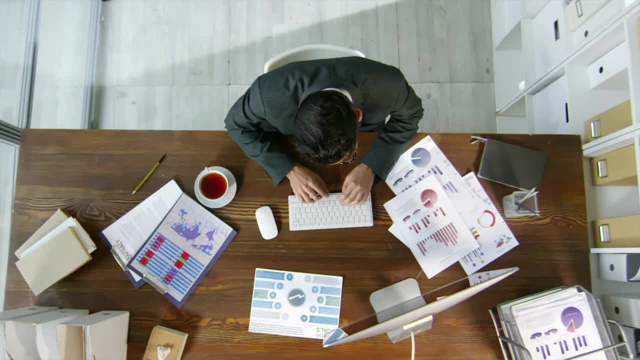 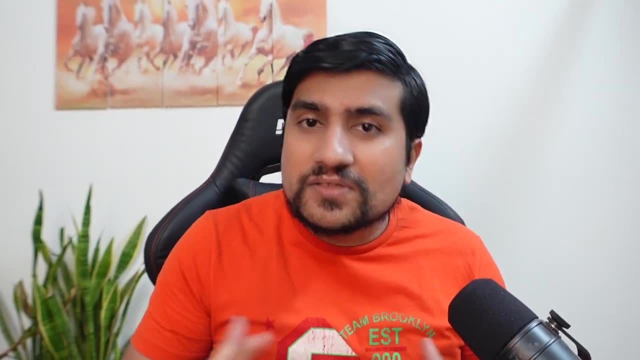 mentioned into the test strategy Schedule. What exactly is the schedule of this overall project that we are going to mention? What are the risks involved? Exit time, grid criteria, How the bugs will be there, How. what exactly is the definition of critical bug and non-critical bug? You have to 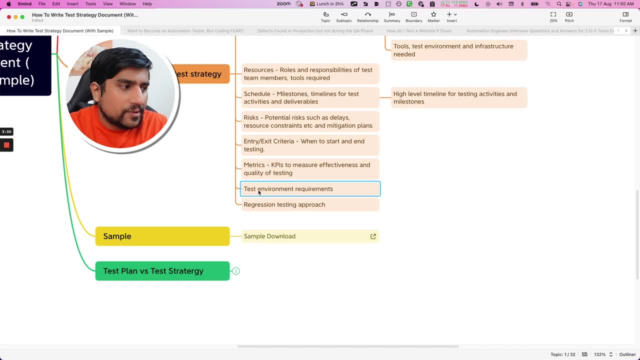 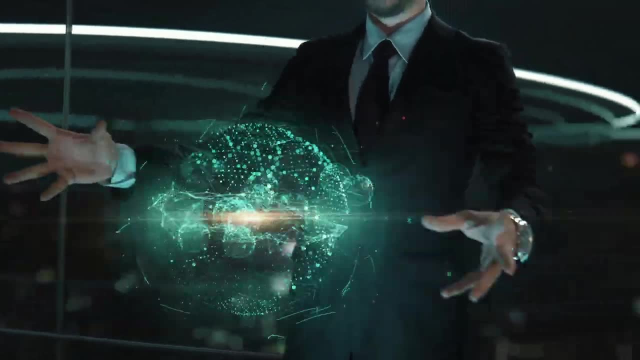 give definition in the test strategy, Regression approach and test environment setup and everything right. So now let's see some sample, right? So this is going. I'm going to show you first of all, very advanced kind of test strategy which is maximum time I have seen people are using in very good. 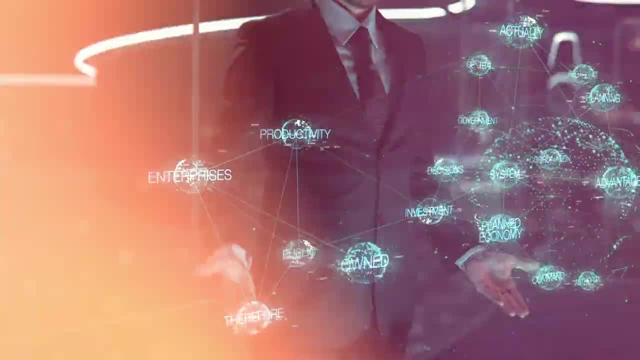 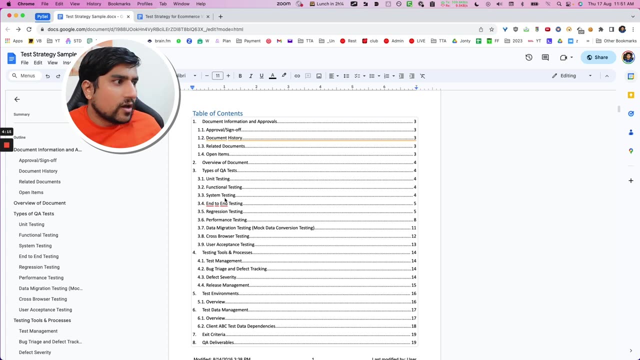 like, I think, CMM 5 level and multinational companies like, for example, Infosys, Wipro, Ascensio, right, I have seen this. So this is a test strategy template from there. If you notice, it's a very big one which contains who is going to approve. 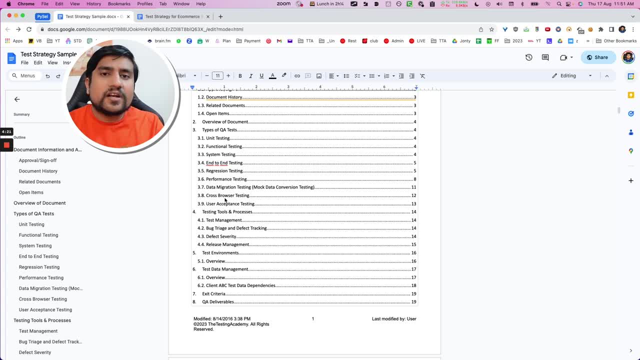 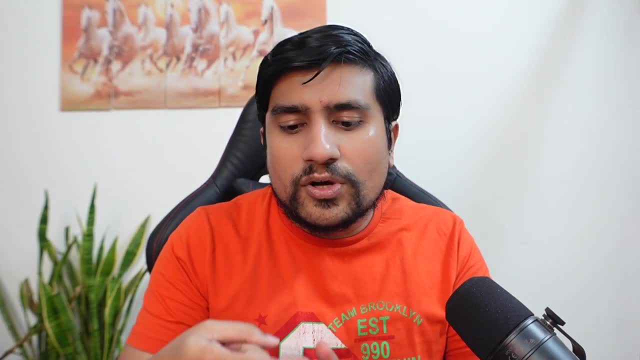 What type of testing you are doing, Test tools, Test environment, Exit criteria. What are the deliverables? Test release: How release happens. What is your devet strategy? Which tool you are going to use? right, So it mentioned what, how, when, who, all these questions in this case. right, If you? 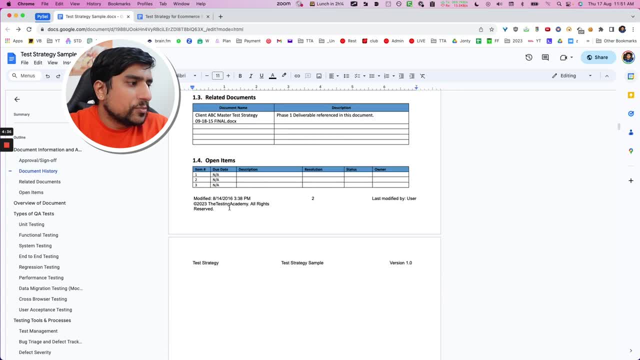 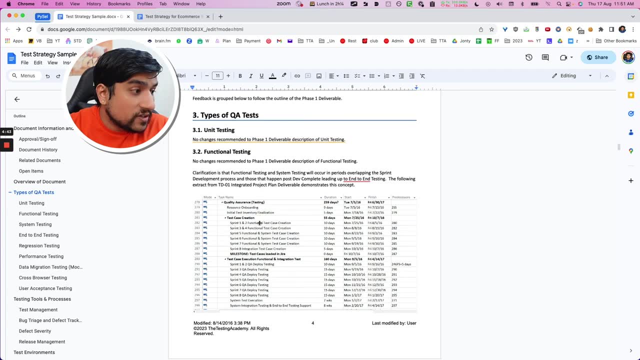 read more about it. right here you can see that who is going to do the approvals right. What are the type of different type of testing we are doing in the unit? For example, unit testing we are doing right. We are doing functional testing, How the sprints will be done in case this is a 10 day. 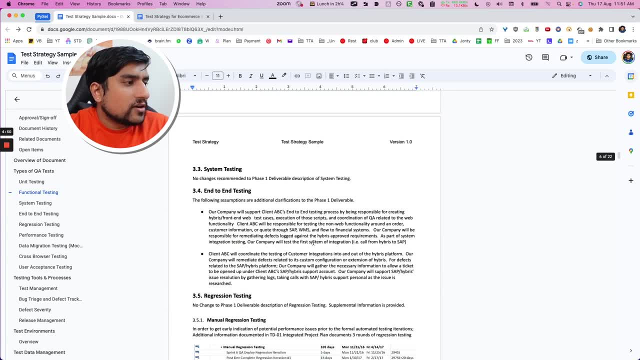 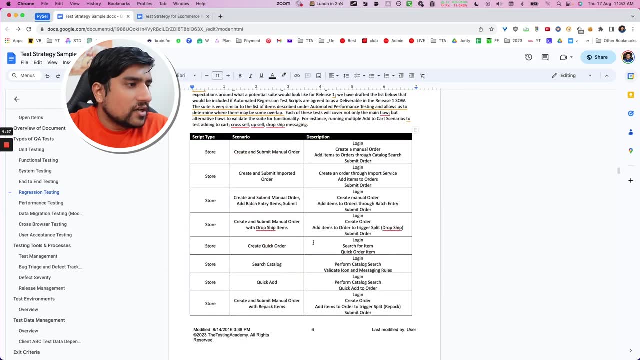 sprint. This is going to be a 10 day sprint. All these are going to. they are going to mention what testing approach, What is your regression approach, How manual regression is done, How automation will be done, How automation testing, Which part of automation will be done, Everything. 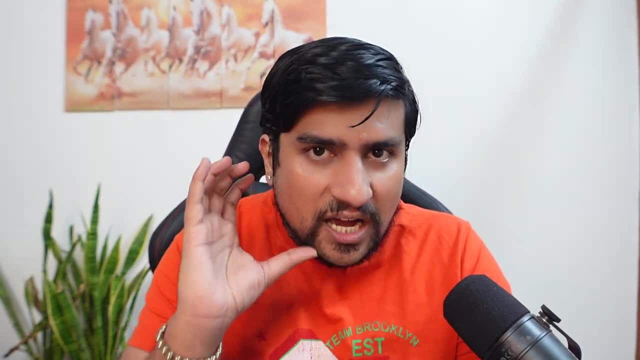 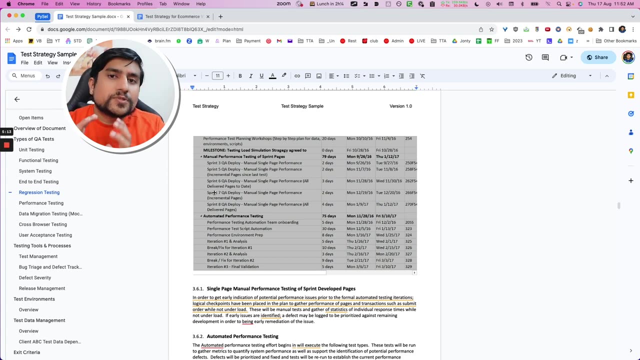 they are going to mention in a very high level manner- High level, Not in depth. High level manner. they are mentioning everything. Note this If you are doing performance testing here. they have mentioned which scenarios they are, Which type of sprints, How this performance testing is done. 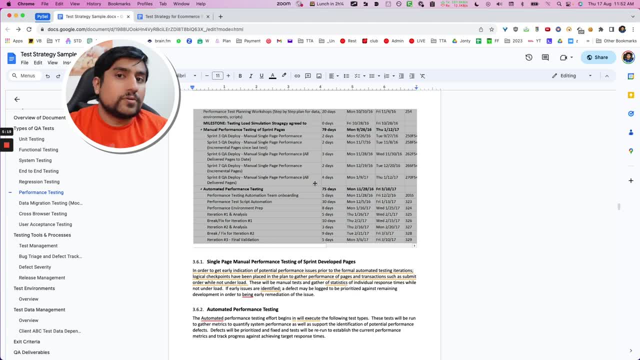 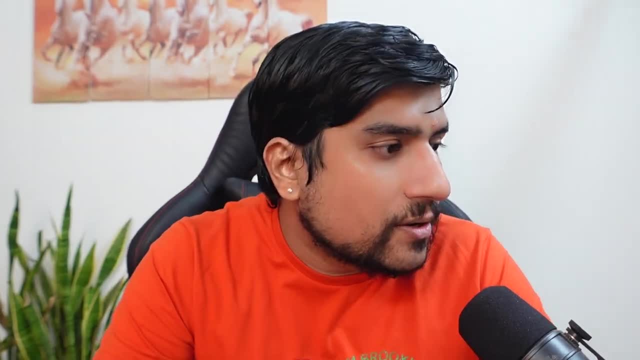 Which sprints they are going to do, How much time it will take. also, they have also mentioned- if you see right, It is so in depth, right, It cleared how and what, clearly, When you are going to execute everything they have mentioned here- How automation of performance testing will be done. 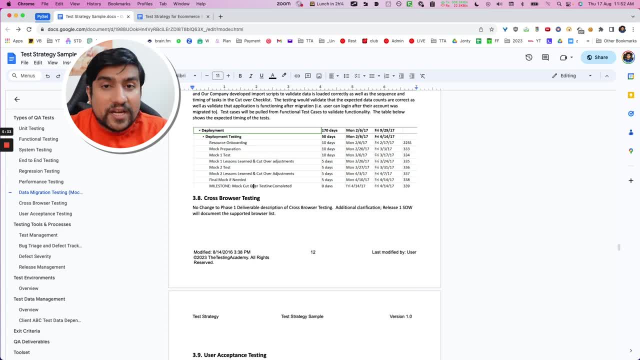 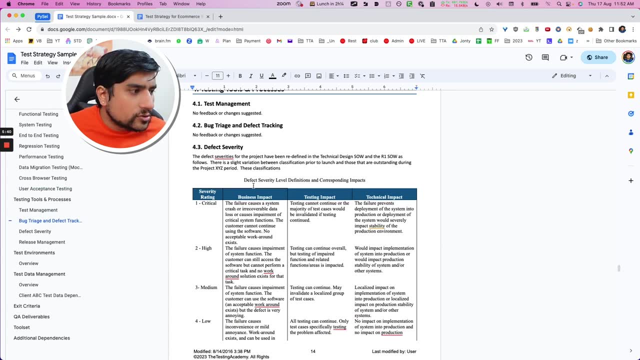 Everything they are going to mention: Browser based data migration. If migration is allowed, Migration requires Cross browser testing is required User acceptance testing, which is UAT. Which tool they are going to use? So they are going to use Jira with Zephyr. 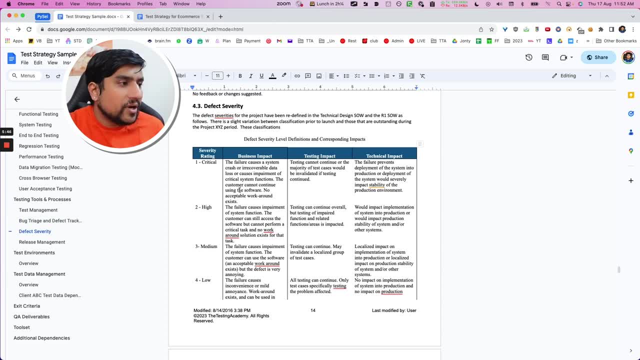 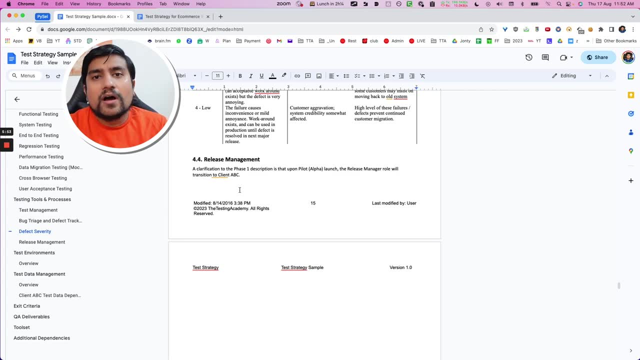 Right, What is the definition of the bugs? right, Critical, high and medium, Everything. in this case, they have mentioned critically How release will be done. For example, there will be alpha release, then beta release, Then there will be overall release, Everything they are going to mention. 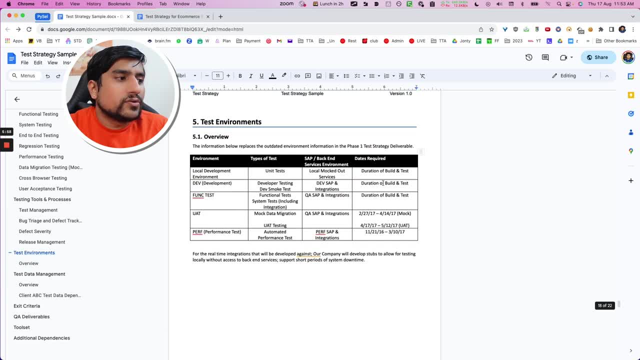 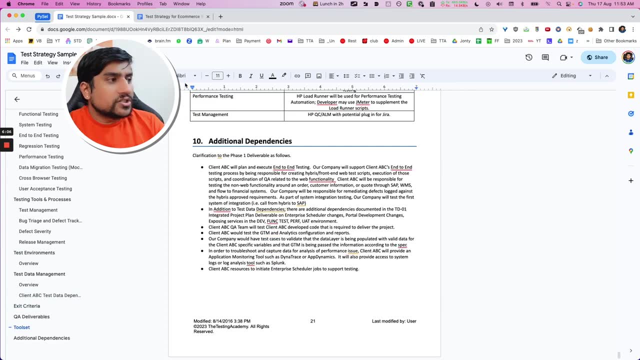 They have mentioned. this is the environments they are going to use, When they are going to use Which data is required. Everything in the table, if you see, are required: Exit criteria, Toolset, additional in this case, right, So this is a very big one, But again there is a one lighter version. 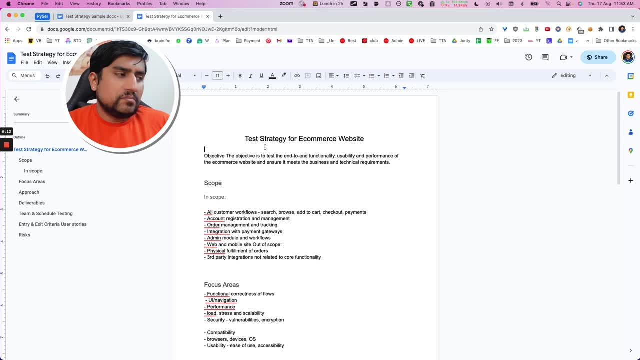 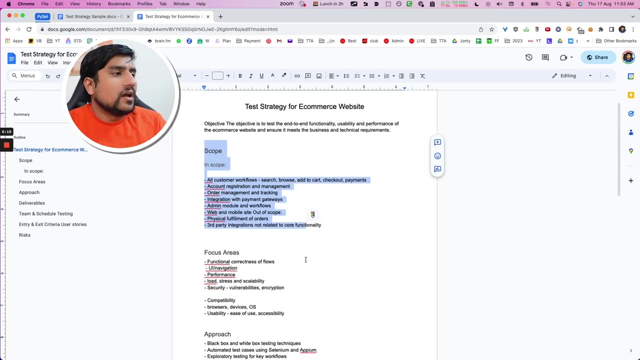 also which I have personally used, And this one is we have used in multiple startups right Where we have seen test strategy directly. they are mentioning all the scope. For example, what are the scope for customer flows that we have? Focus area approach: How you are going to create your test. 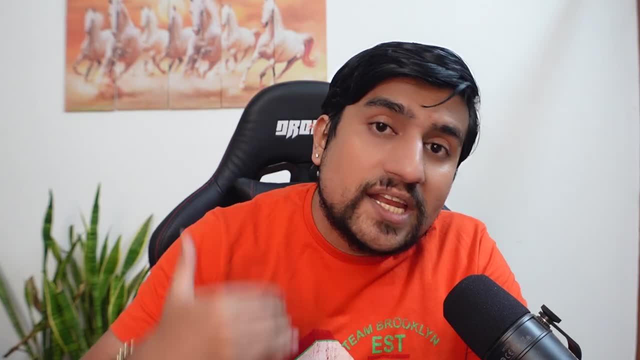 cases, For example, boundary value Equalization. How you are going to create your test cases, For example, boundary value Equalization. How you are going to create your test cases, For example, boundary value Equalization, Length partition. How you are designing your test cases. Everything you have mentioned, Which. 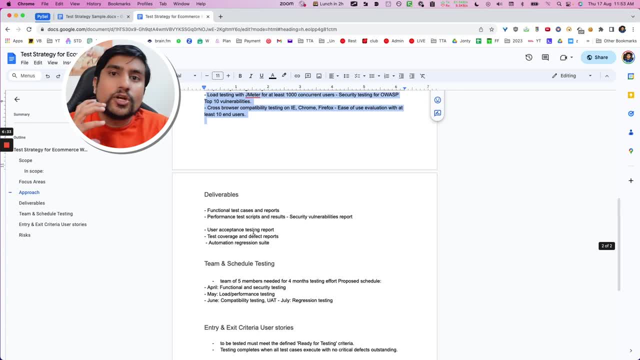 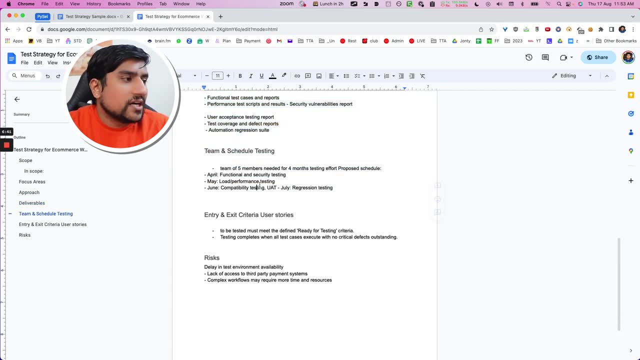 automation you are going to use, How you are going to do lot testing and everything With the schedule you can mention. What are your deliverables, Test closer, report Everything you are going to mention here. What will be your regression time and scheduling time? Four months time it will take. 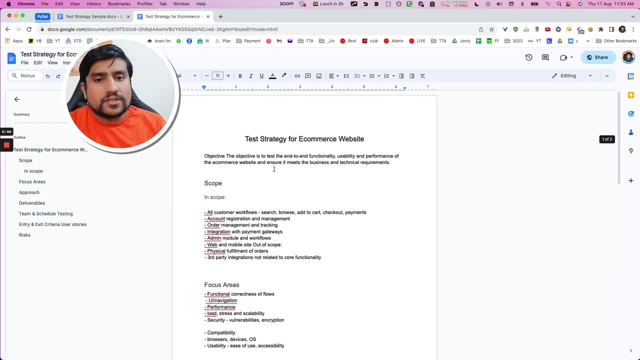 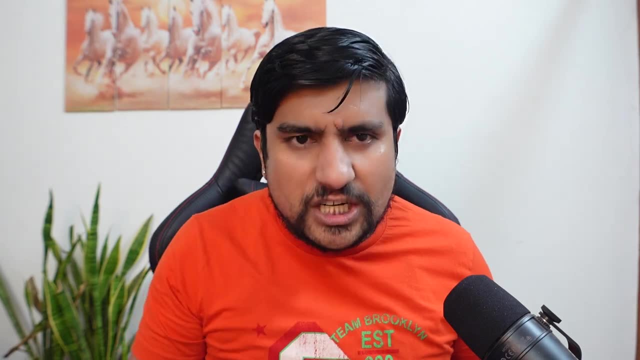 Exit criteria, risk and everything. Second one is a lighter version on this right. I hope now this is clear. how to create a test strategy from the scratch. I am going to share both of the link in the description. You can check it out. You can copy this and use it in your project also, okay, 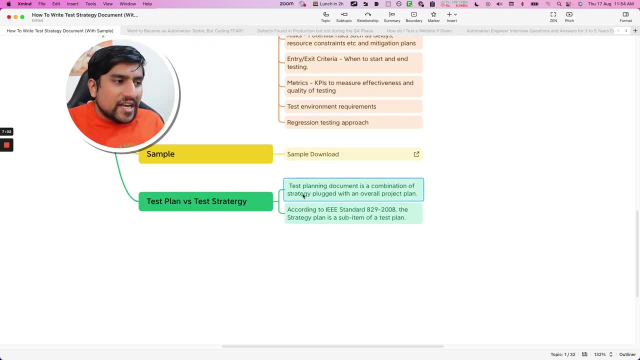 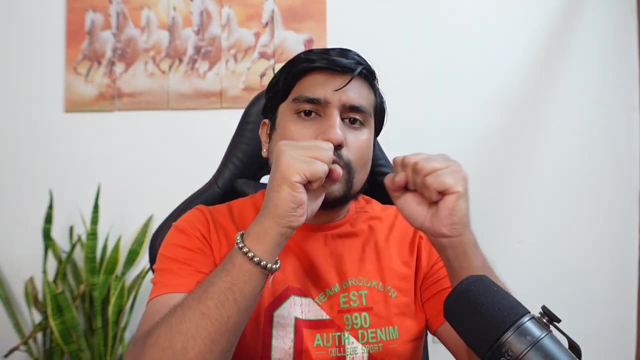 Now the main interview question, which is test plan versus strategy. Test planning is a combination of strategy plugged with the overall project plan, right? So test plan, if you see right, It is basically test strategy plus project plan, So it's a bigger version of it, right, Overall, if you see? 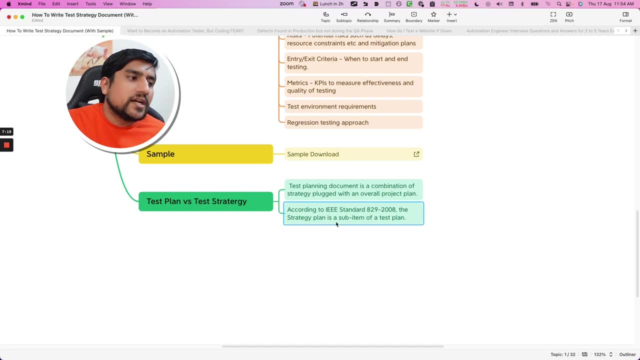 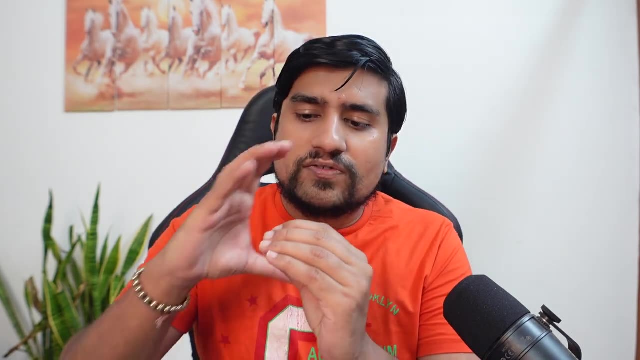 right. Test strategy is actually a subset of the test plan as per the IEEE standard 829 and 2008.. So many people actually don't know, But test strategy is actually but nothing but a smaller set of your test plan. It's a smaller set of your test plan. Test plans also include project plan. 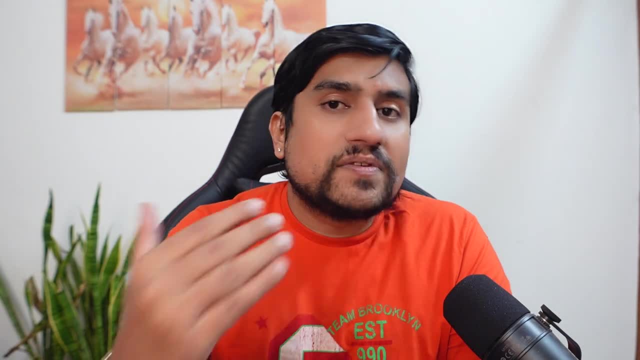 and other things also in this case, right. So I hope this helps. If you liked this video, please subscribe to my channel And test plan also. I have explained in another video. You can check it out. This is a very in-depth video where I have created for test strategy. I have shown you two.